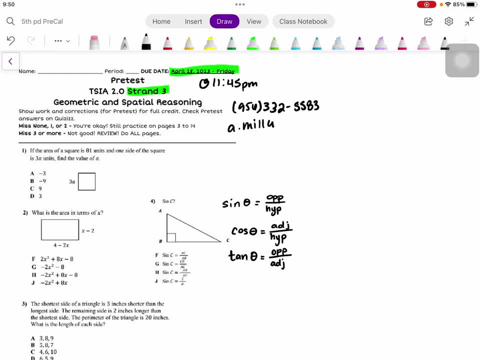 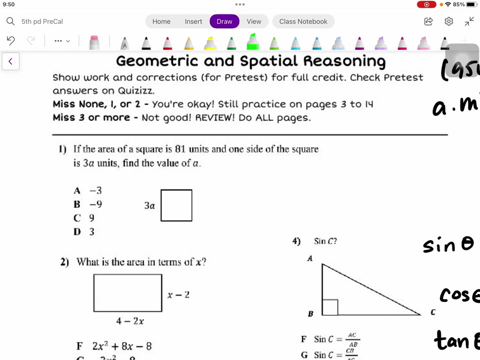 voice number Or you can email me just in case you have any questions. okay, All right, so let's go into the instructions. So make sure you show your work and, of course, the corrections for the pre-test for full credit Check, pre-test on answers on quizzes, right? So if you do number one, 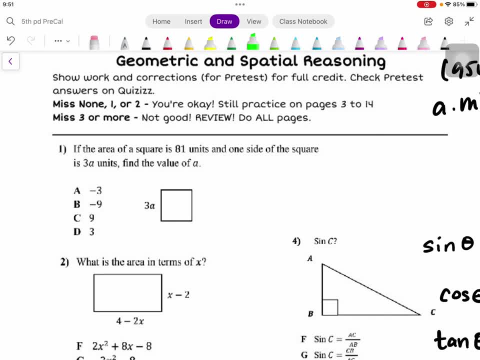 you put the answer is E, Then if the answer is not E and then it turns out to be D, then you need to write down the corrections from this video. okay? So if you miss none, one or two, you're still okay. You still need to practice on problems or pages three to 14.. If you miss three, 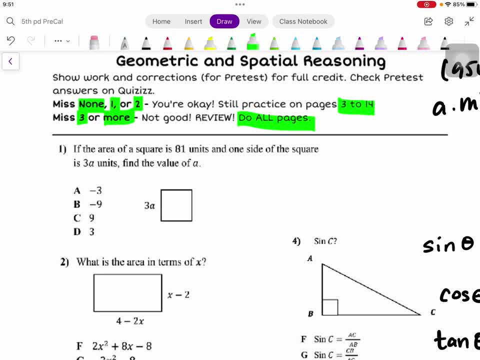 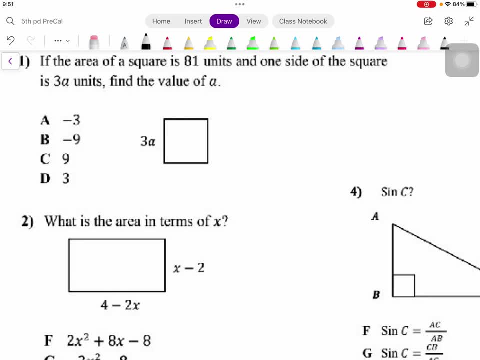 or more. it's not good, So you're going to have to do all the pages right, So be very careful when inputting this onto quizzes. So let's start with number one. So if we have the area of a is 81 units and one side of the square is three A units, what is the value of A? all right, So. 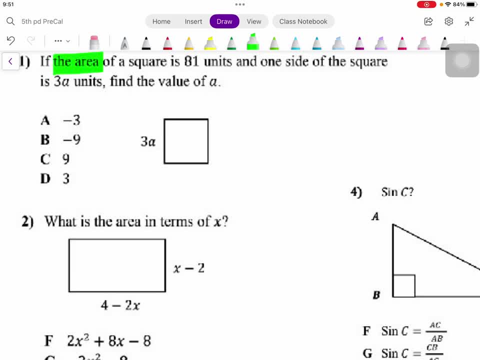 let's go ahead and highlight some things. So we're saying that the area of the square is 81 units. we don't have a specific like feed or anything, so we're just going to call it 81.. Now, one side of the square- all right, so it is a square, is three A units, all right. And then 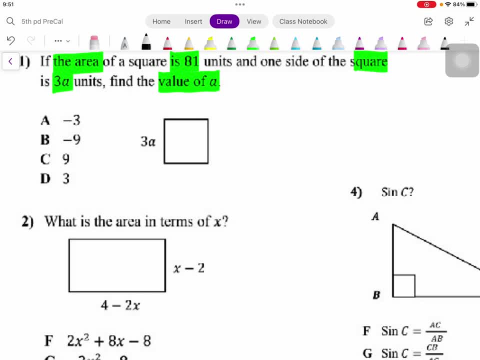 we're trying to find the value of A. Now, when we are given the value of A, we're going to find the value of A. a square that means we have: all the sides are equal to one another. So since one of the sides 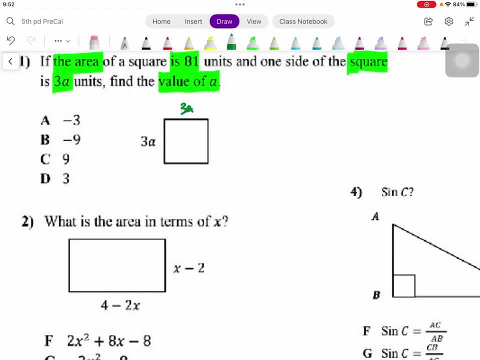 is a 3A. the other side, right here, is also a 3A. Right across from here, is 3A, and this one's all 3A. So all the sides are equivalent to one another, right? They're all congruent to one another. 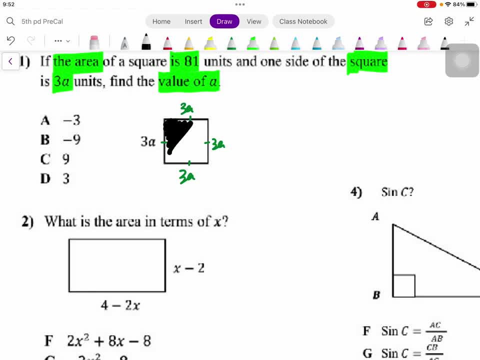 Now the area of the square, this whole entire area is actually 81 units right, So all in total 81.. So how are we going to put that in an equation? Well, the equation for a square or a rectangle to find the area is: area equals length, right That's an L times. width, right, Length times. 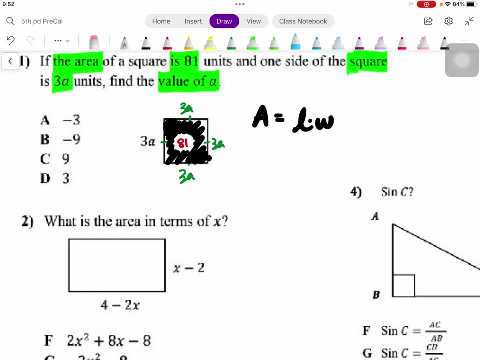 width. So my length in this case is 3A and my width is. the other one is right here also, okay, So now I'm just going to go ahead and insert it, So it's going to be 3A times 3A and that's going to equal. 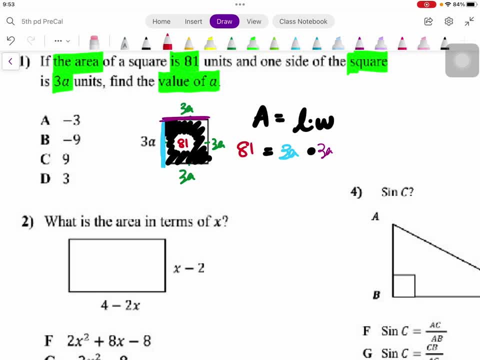 in total the area, which is 81, right. So now that I input that into my formula, I'm going to have 3A times 3A and that's going to equal, in total, the area which is 81, right. So now that I input that into my formula, I'm going to have 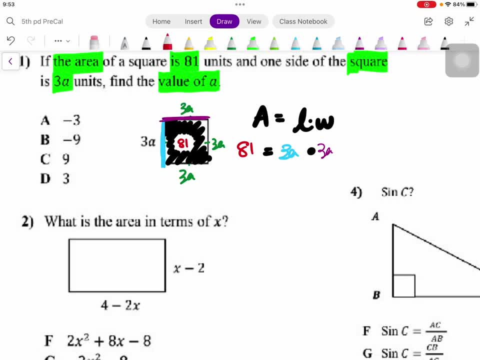 to solve for A right, Because we're trying to find the value of A, which is just a number. Now, to simplify this, we're going to do 3A times 3A. Well, 3 times 3 is a 9.. A times A is A squared. 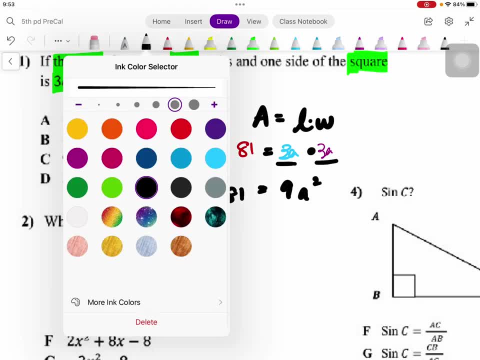 and that's going to be equal to 81.. That one didn't get messed with, so we're just going to leave it as 81.. Now what we need to do is to get A by itself, So we're going to get rid of 9 first. 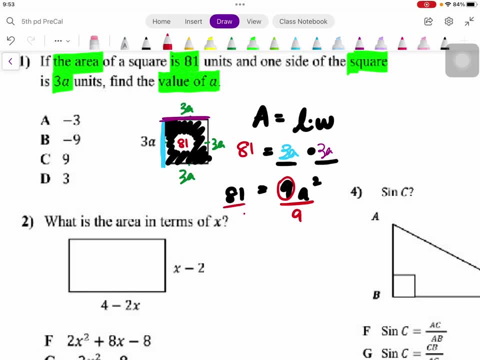 So the opposite of multiplication is division. Divide 9 here, divide a 9 here, and then, of course, if I rewrite it, it's A squared is equal to 9.. Now I need to get A by itself, so I'm going to get. 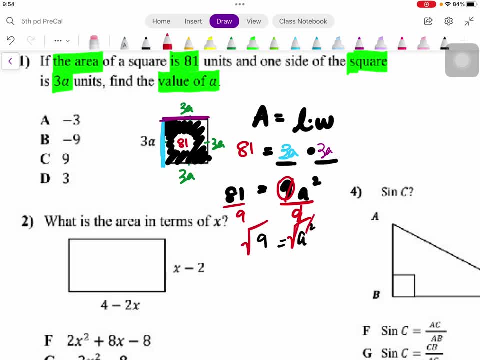 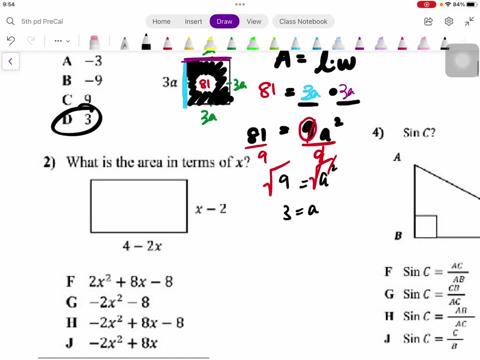 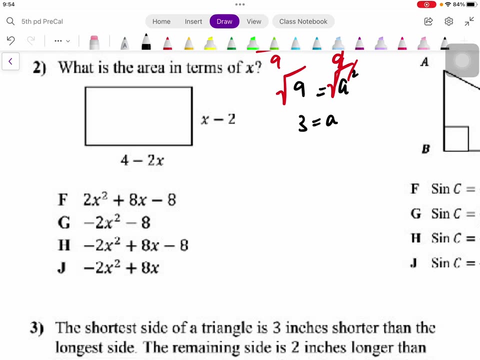 rid of that square by square rooting it. What I do to one side, I do to the other. Square root of 9 is a 3, and that's equal to A. All right, now for number two, same thing. What is the area in terms of X? So this type of shape? 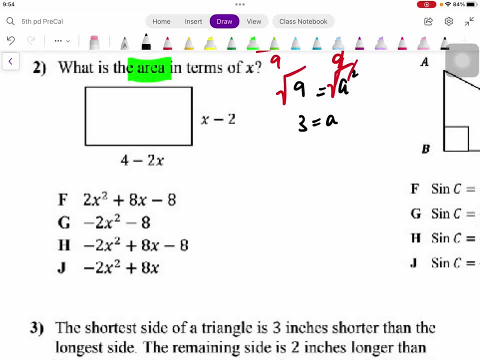 is called a Rectangle, which is the same formula. So area is equal to length times your width, right? So it really doesn't matter which one's length, which one's width- This one right over here, 4 minus 2X. 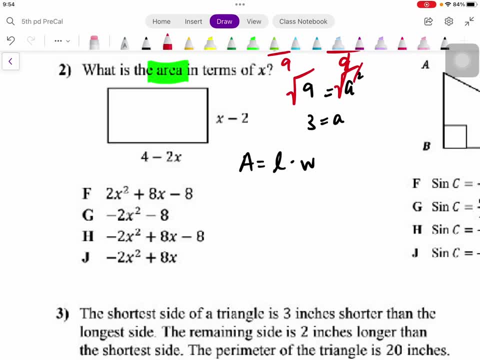 you could put that as a W, you could put that as an L, It really doesn't matter, It's still going to be giving you the same thing. So I'm going to put that one as width and then this one as length. 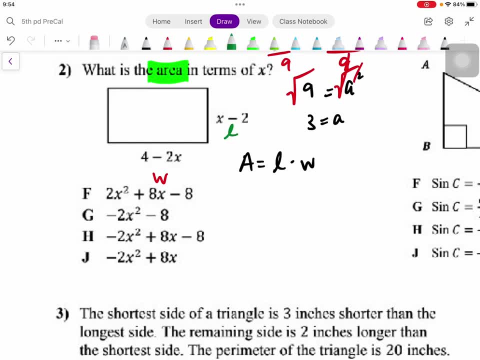 Now I don't have area this time, so I'm actually going to evaluate or I'm going to not evaluate, sorry. I'm going to simplify By just taking L and multiplying with W and then calling it quits, right, So my L is going to be X. 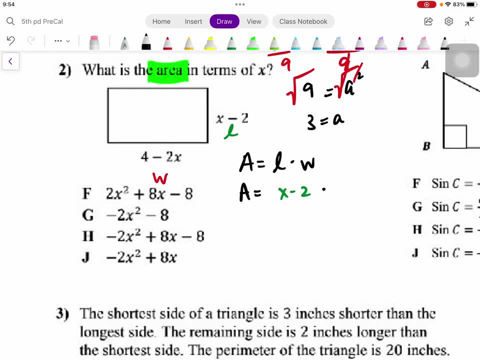 minus 2, and that's all going to be multiplying 4 minus 2X. Now notice: each one of these- one in green and one in red- have more than one term, meaning that you got X and minus 2, and then you. 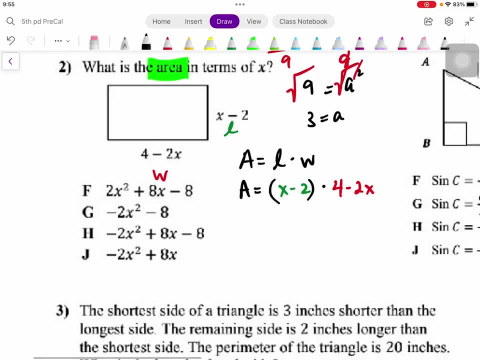 got 4 and minus 2X right. When you have more than one term, your best bet is to put it in parentheses. All right, so here we're going to multiply. So, since we have more than one term in each one of, 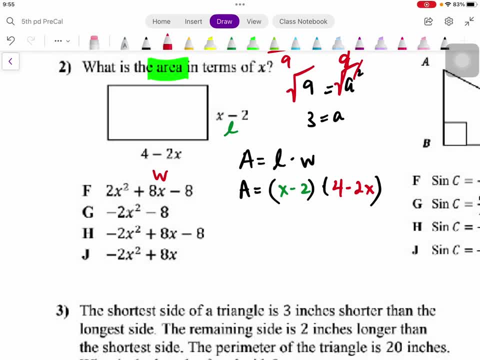 those, we're going to have to do a special type of distribution which is called the FOIL method, right? So we're going to take the first one. with the first one, 4 times X is 4X, and let me do that in black. We're going to do FOIL 4X and then we're going to do X. 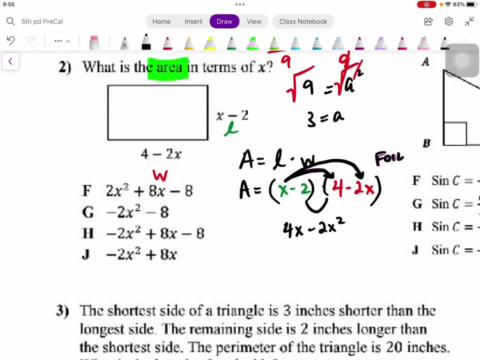 times negative 2X, which is negative, 2X squared, and we do negative 2 times 4,, which is negative 8.. Negative 2 times negative. 2X is positive. oops, positive 2X, right, And of course now you have. 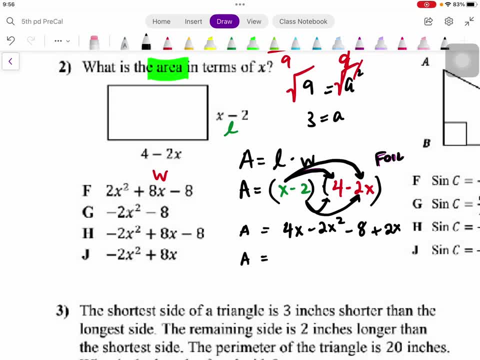 to combine like terms and of course, you want to do it from largest power to the smallest power. So the small, or sorry, the largest power happens to be a 2.. So I'm going to take this term and I'm 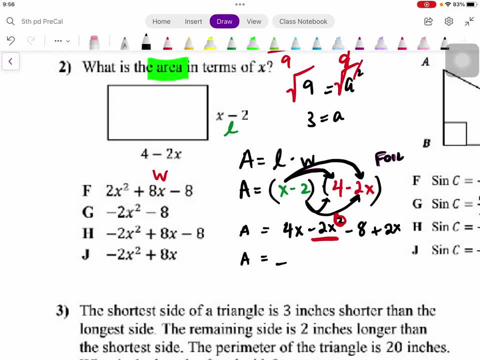 going to write it down because there's nothing else to combine it with, So I'm going to write negative 2X squared. Next we have the Xs, 4X, and 2X gives me 6X, and the last one is the constant, which is negative 8,. 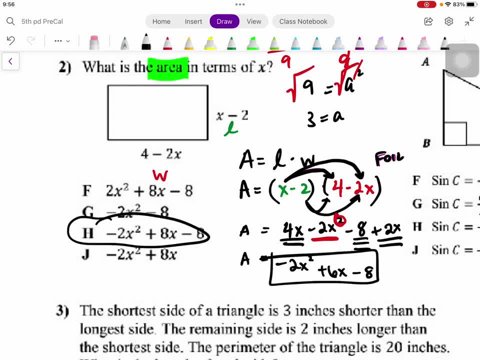 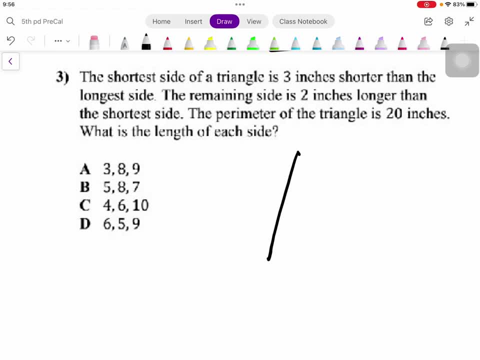 right, And then that should be my answer, which is answer choice H. right, So moving on to number 3.. All right, All right, so the shortest side of the triangle is 3 inches shorter than so: 3 inches shorter. 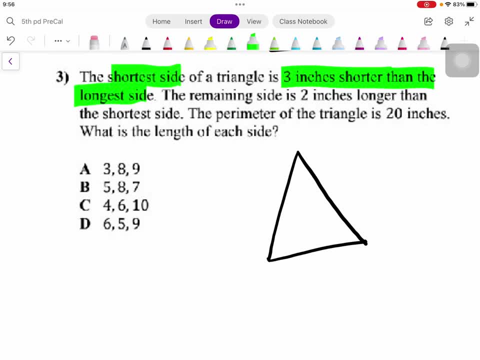 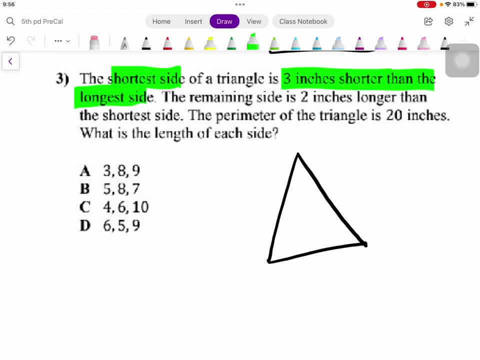 than the longer side right. So this is the shortest side, and the remaining side, which is not the long side or the short side, so it's the one in between- is actually 2 inches longer than the shortest side, So it's just a little bit bigger and then smaller than the longer side. 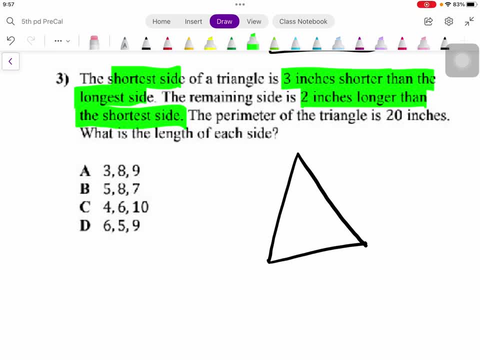 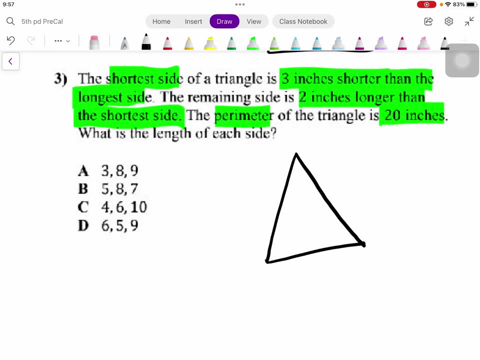 right, So the perimeter of the triangle, all around, right, So perimeter of the triangle is 20 inches. What is the length of each side? All right, So perimeter means we're just adding up all the sides. So we're just adding up all the sides and then we're just adding up all the. 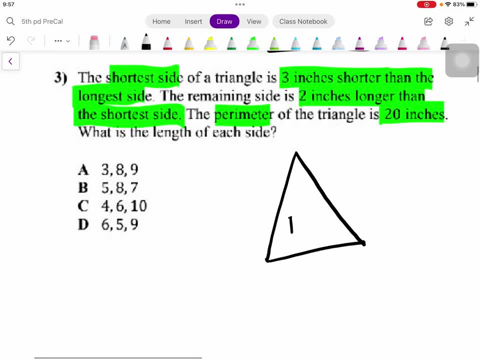 sides to one another and it should give us a total of 20 inches. So I'm going to put P is equal to 20.. Now, it doesn't matter which one's your short side, which one's your long side, because this is just a simple illustration, right? So we don't know what the long side is. 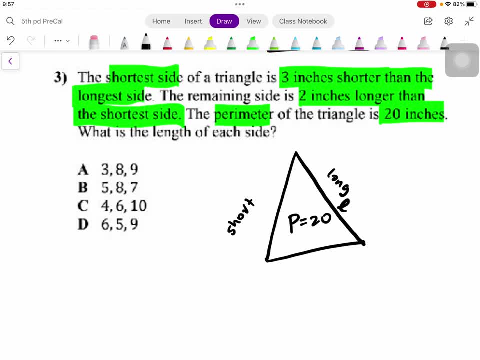 right, So I'm just going to call it an L. but they are saying that the short side is 3 inches shorter than the long side, right? So I'm going to put P is equal to 20.. So I'm going to put P is. 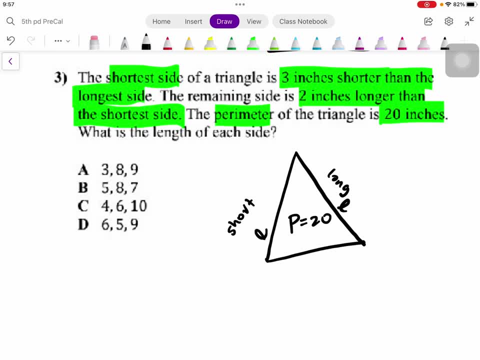 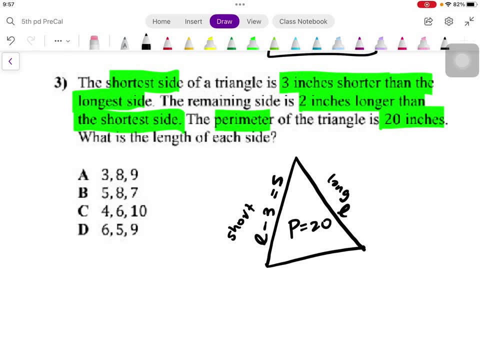 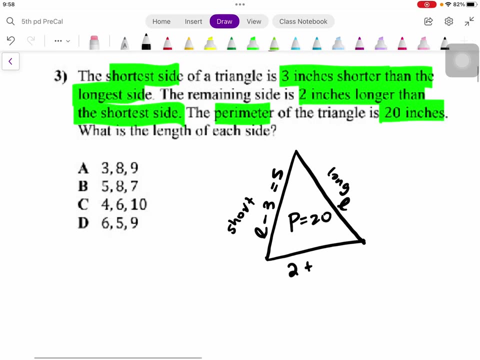 equal to 20.. So I'm going to take the long side and I'm going to subtract 3 inches to get the short side, So that should be equal to RS. Now the remaining side, which is the in between the short and the long, is actually 2 inches longer than the short side, So I'm going 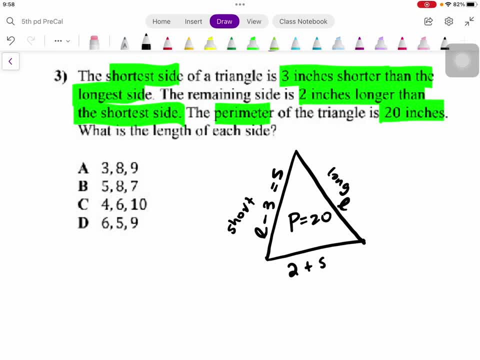 to do? or sorry, short side, All right, So 2 inches longer than the short side, okay? Now, when you're doing perimeter, all you have to do is add up all the sides, So I'm going to put P is equal to 20.. 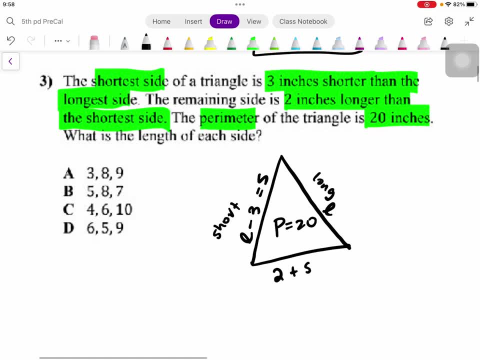 So let's start with P equals. oh, not P equals, right? Well, yeah, Okay, Your P, which is your perimeter, is 20 inches, is equal to your short side, which is L minus 3, right, We're not going. 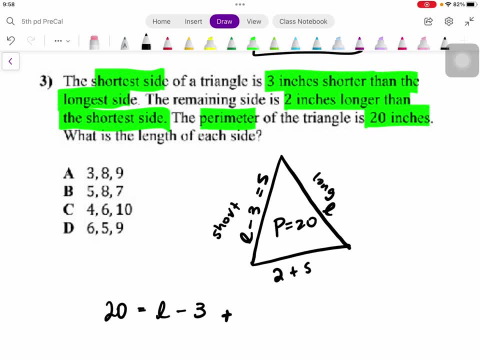 to include the S, And then we're going to add that with our long side, And then we're going to add that with our remaining side, which is L minus 3, right, So we're going to add that with our long side, which is 2 plus S. right Now, you're more than welcome to put parentheses, but we're 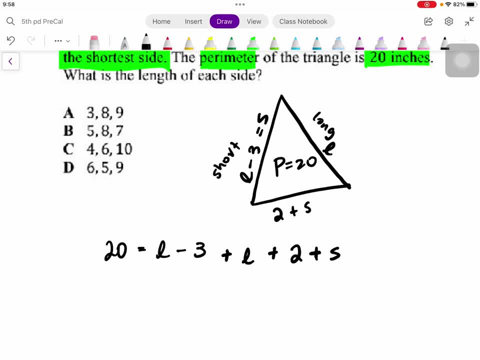 not multiplying here. So you don't need to put the parentheses, if you know, because with addition it doesn't change the signs. So it's okay to not put parentheses. It's only okay to put it when you're talking about area, All right. So now we want to put these in terms of L, right, Because 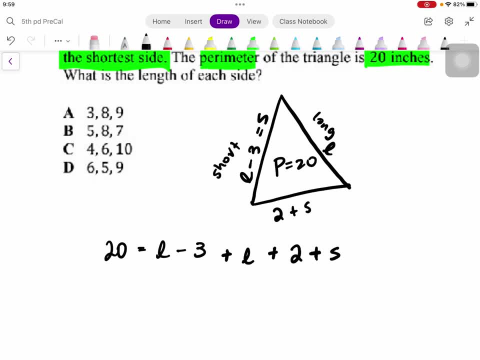 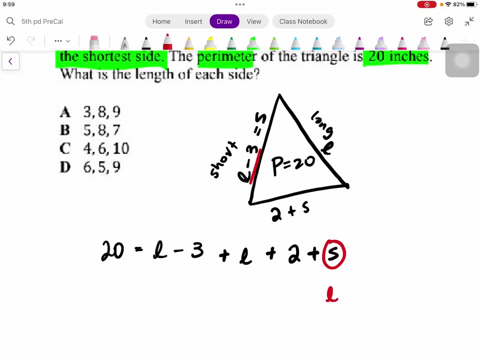 we're going to have to solve for one letter, And I see that there's already two L's. Now S, I know S, which is our short side, is also also known as the long side minus 3, right, So I can replace that S with long side minus 3.. And 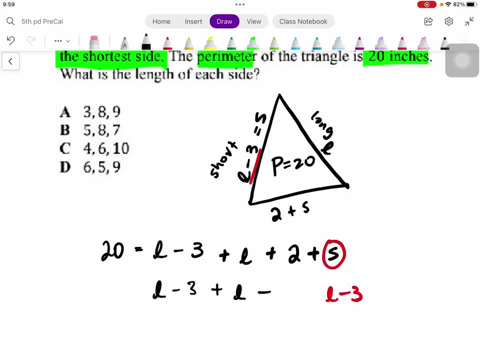 then I could just bring everything else down. Now that I have everything in terms of L- because I'm going to have to solve for L to determine what each side is- I can go ahead and proceed on. So I'm going to combine like terms. So let's start with the L's. So I got one L, two L's, three L's. 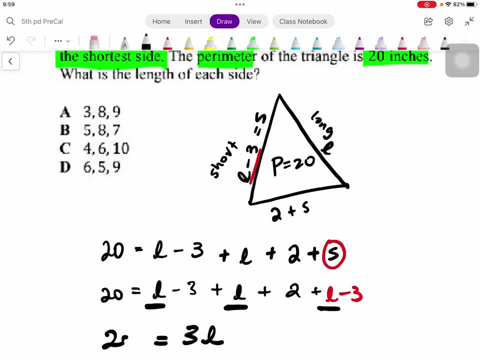 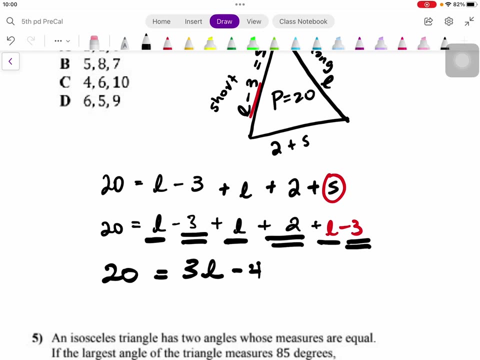 So I have three L's, All right, And now we're going to combine the numbers together. So we got negative three plus two, which is negative one. negative one minus three is the negative four. Now, now that it's more simplified, you want to solve for L, So I'm going to get rid of the four by adding four to 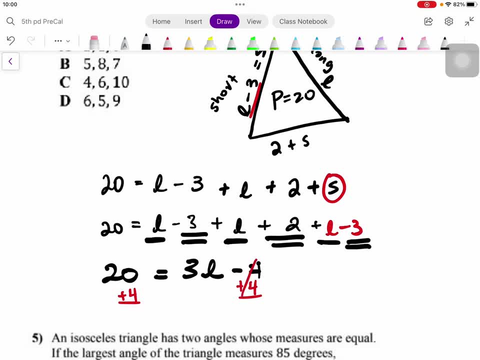 both sides. 20 plus four is 24.. Let me rewrite it over here: 24 is equal to three L. Now three times L are multiplying, So I'm going to have to divide, And 24 divided by three happens to give me an eight, an ocho. 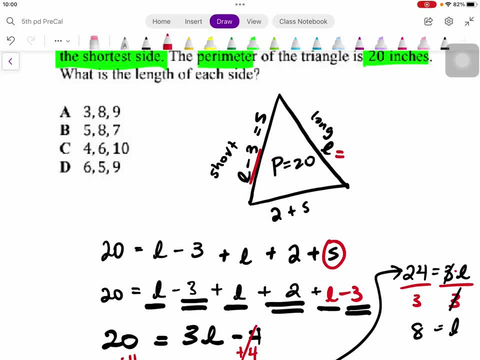 right, So I already have my long side. Long side automatically is eight. Now for short side. you're taking your long side subtracting three and you should get your short side, which is a five. So you're going to look four sides as five and eight. Now I know I can cancel out A because 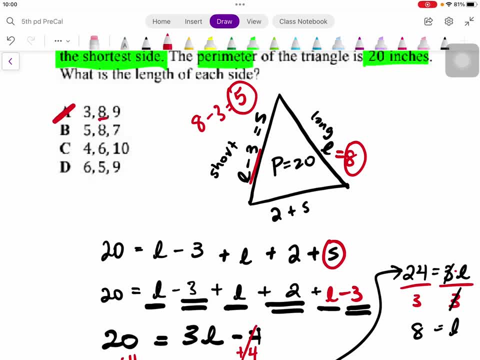 it has an eight, but it doesn't have a five. Possibly an answer, because it has a five and an eight. C doesn't have an eight, neither does D, So your answer is going to be B, but let's just continue on to see if that last side is going to. 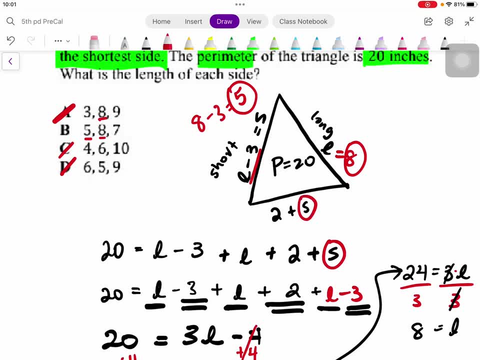 be seven. Well, short side is five And of course, if I add two, that is going to give me seven. So indeed, B is your answer. Okay, All right, moving on. So let's go on to problem number four. Problem. 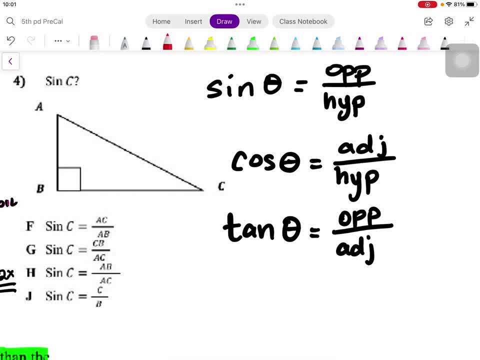 number four requires us to go back into geometry and look into our trig. I know some of you guys did not do trig, which is perfectly fine. It should be. hopefully it won't be too hard to understand. Now, here they're asking for sin C. Some of you guys are like: what is sin? Well, 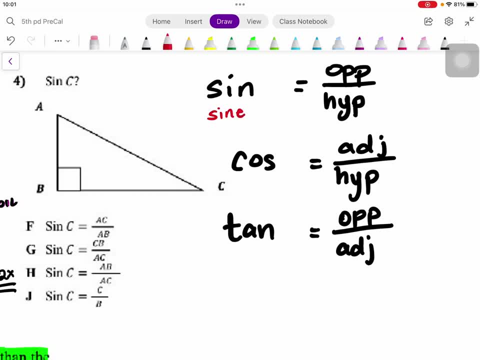 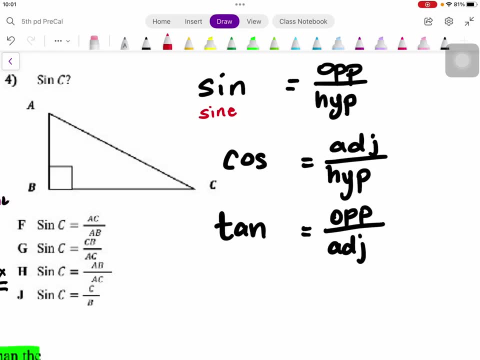 it's not actually called sin, It's called sine, It's just abbreviated. They just don't include the O, They don't include the E. So when they say, when you see sin, it really means sine. If you see a cos C-O-S, that actually means cosine, And if you see a tan, you're not doing. 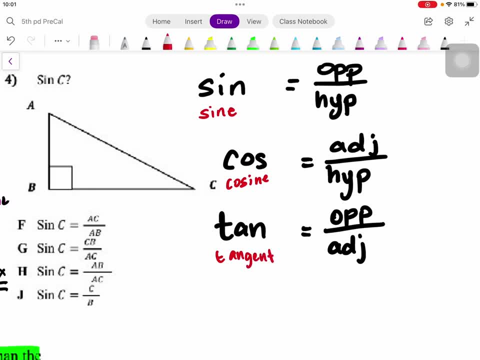 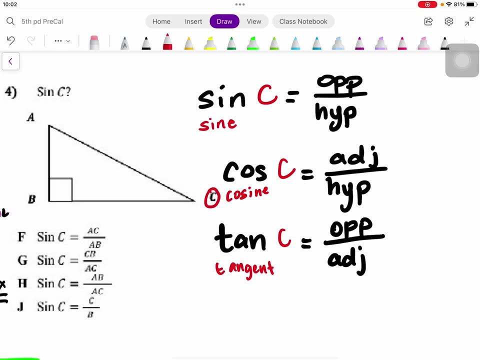 a tan. It actually means tangent right, It's just abbreviated. Now they're asking for C. So the reason why I erased those thetas is because we're going to look at different sides from a specific view, which is at angle C. Now here's point C. The angle C is right over here. Now why am I saying? 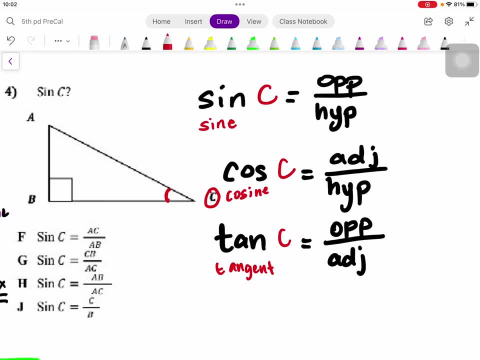 at a specific spot. Well, we can look at a specific spot. Let's say we're in a tree right And the tree is angle A right, Looking down. you're looking side to side. That's a different view. But if you're looking 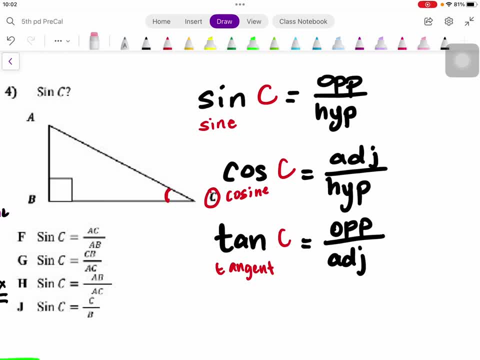 here in the bottom, such as C. you're looking at it from that point of view. okay, Now each side is going to be different anytime you look at a specific angle. So for here, for instance, for angle C, it has different sides. So what you're looking for is that you want to look for. 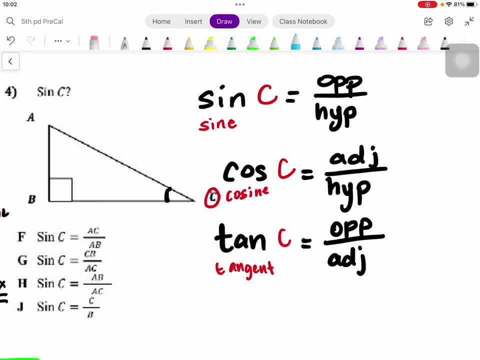 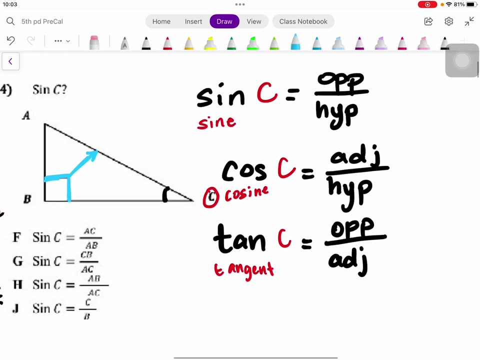 the side and adjacent side. Now the easiest one to spot is your hypotenuse. Hypotenuse is always opposite of this little box. That's a right triangle or right angle- sorry, right angle- And opposite side- right Opposite means across- is going to be your hypotenuse. Now, sometimes you 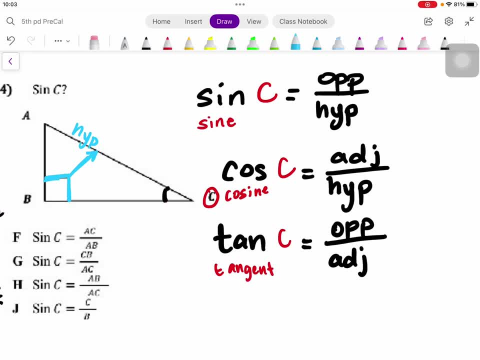 might see me abbreviate as H or HYP, just because it's a really long thing to write out, right? So this side of the triangle is called the hypotenuse. Hypotenuse Now for angle C, for opposite side. according to this, C opposite side is opposite. 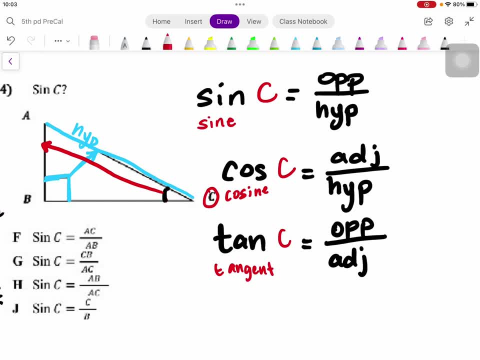 of this angle, just like that box, And this is going to be your opposite side for C. So OPP or O is fine. Now the last one, adjacent, means next to. So what's next to angle C right is going to be your hypotenuse. So what's next to angle C is going to be your hypotenuse. 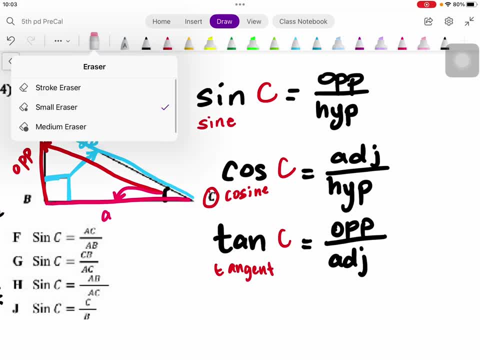 I probably shouldn't have put it in pink. Oops, All right. All right, So this one in yellow right, This is our adjacent side, which you abbreviate it as A or ADJ. So that is listing out or labeling the sides right From angle C, Angle A is different. All right, So now what? 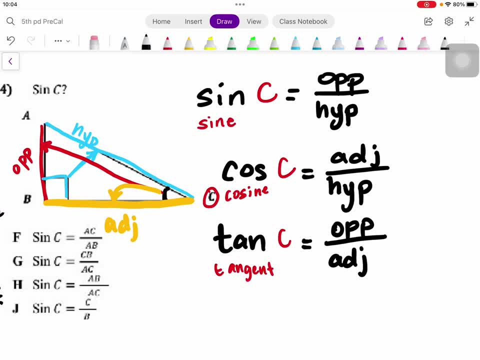 they're looking for is sin AKA sign. So we're going to be taking our opposite side right And we're going to divide it with our hypotenuse. Now, our opposite side right, The one in red, is from the points from A to B. 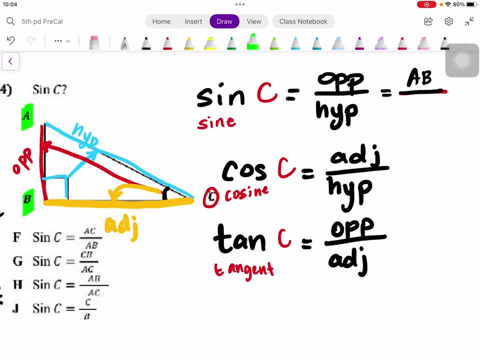 So I'm going to write A to B right over here, And then as far as our hypotenuse- our hypotenuse is the blue one- It's from angle, or sorry, from a point A to point C, right, This whole entire thing. So I'm going to write it as A and C. Now you can. 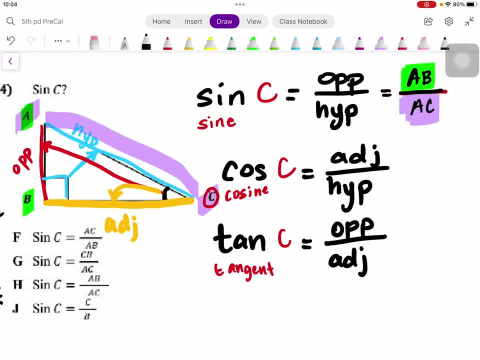 write it as C, A, B, A. It's the same thing, But you're going to see down here below in your answer choices they go in alphabetical order. So my answer for this one happens to be answer choice H, right? Sometimes these problems have actual numbers to it, such as, let's say, this was: 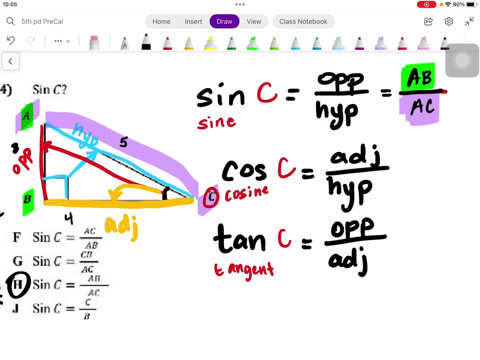 three, this was a four and this is a five. If they asked for A B, then you would put three, And if they asked for A C, which is the hypotenuse, you would put five, And then of. 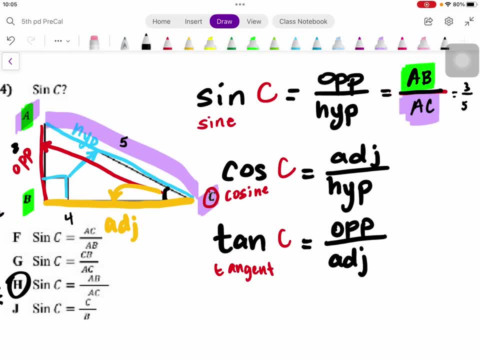 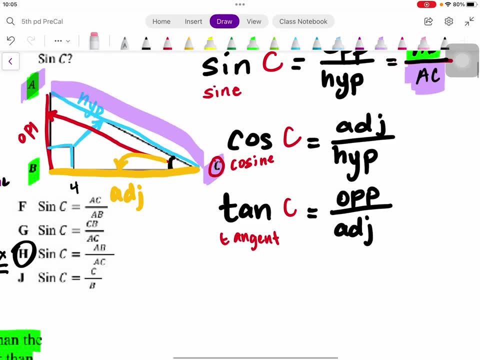 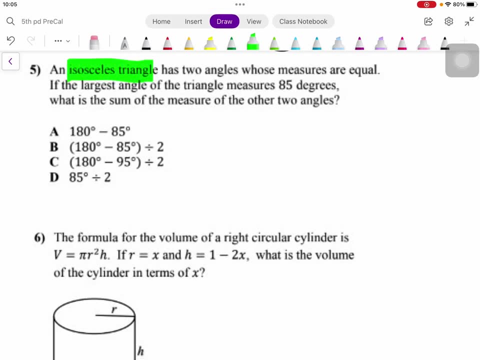 course you reduce the fraction, but three over five is already reduced, So yeah, So that's an extra example for you guys, just in case you have numbers. So let's move on to problem number five. So problem number five is talking about a Sausalese triangle. 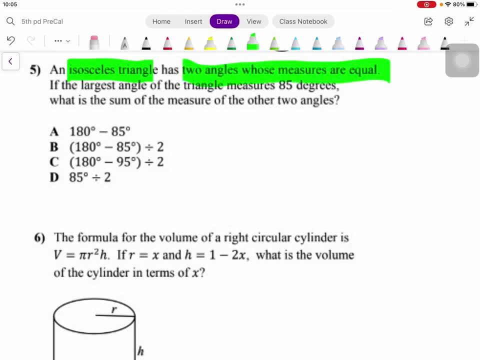 It has two angles. who has measures are equal to one another. If the large angle of the triangle measures out as 85 degrees, what is the sum of the measure of the other two angles? Now notice your answer. choices are not numeral, giving you a value, So let's kind of put an illustration to it. So here, 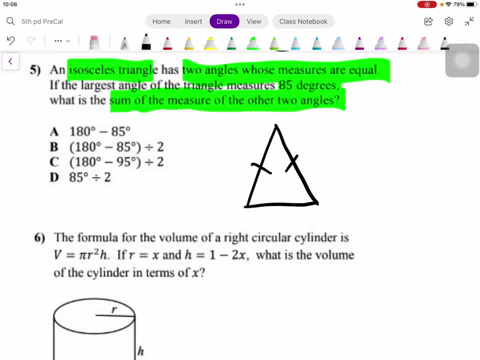 you got a nice Sausalese triangle right. A Sausalese triangle means that you have two sides that are equal to one another. Now, opposite of that, you have two sides that are equal to one another. So, opposite of it right. So opposite of this side right, The angle is going to be same of 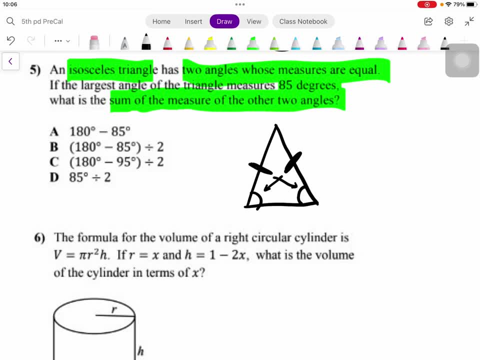 the opposite of this angle, right, Because this angle right over here in red is opposite of this one. And then, since the sides were equal to one another with the yellow one, that means the angle is also the same as the red angle. That makes sense, right? So just kind of think of it as: 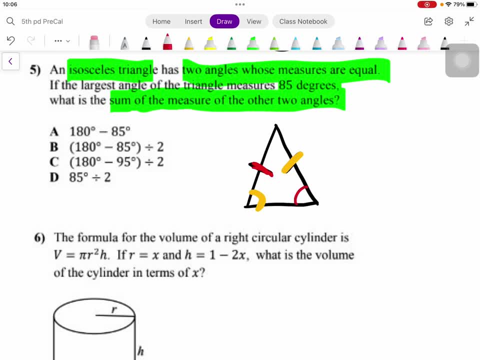 the red angle belongs to this red side and then the yellow angle belongs to the yellow side, And since the sides are equal to one other, the angles are also equal to one another. Okay, Now they're talking about this angle right over here in blue. That is the larger angle, the largest angle They want to know. well, they said. 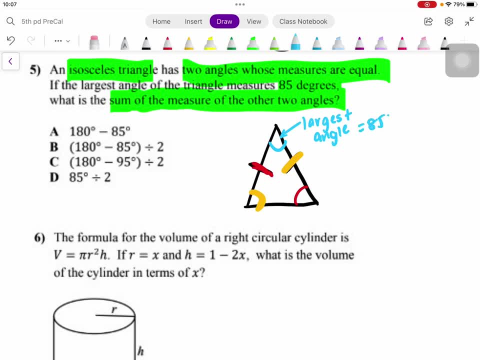 it's 85 degrees, correct. Now, when you add all the angles to one another, to a triangle, it's going to add into the triangle. So it's going to add into the triangle. So it's going to add into the triangle. 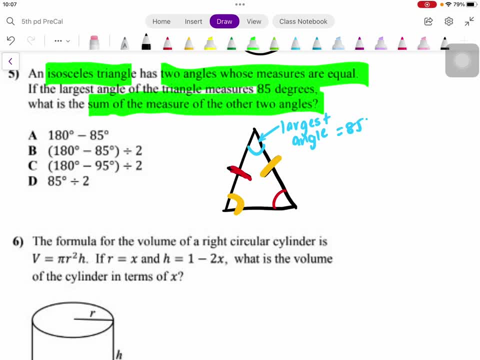 180 degrees. So to figure out what these two are, you're going to take 180, right, And you're going to subtract 85, right, Now, of course, that is going to give us- let's see 95 degrees Now in. 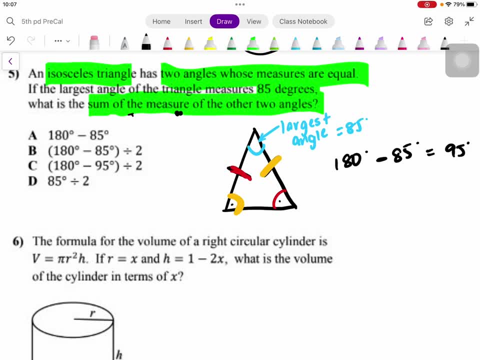 the question. it says: what is the sum of the measure of the other two angles? So they want to know the sum. Sum means addition. So if I add angle yellow, angle red to one another, it should equal 95.. Now I know some of you guys are probably 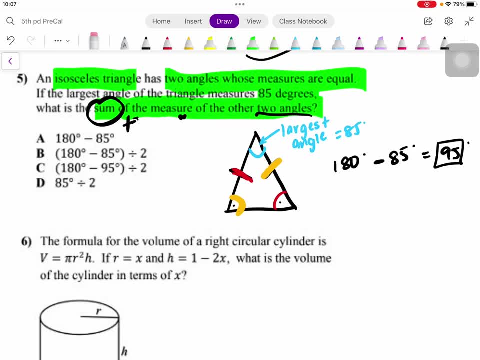 like no, the answer is B. No, that's to find the individual angle We're trying to look for. when we add them up together, it should equal 95. So our answer should be answer choice A. It's all in the. 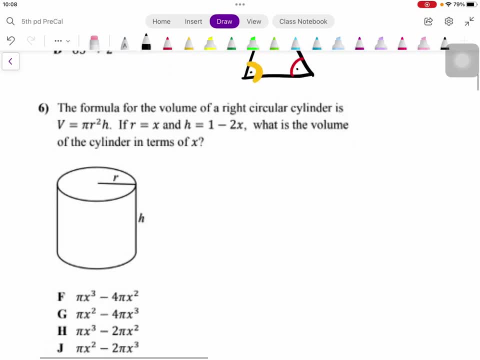 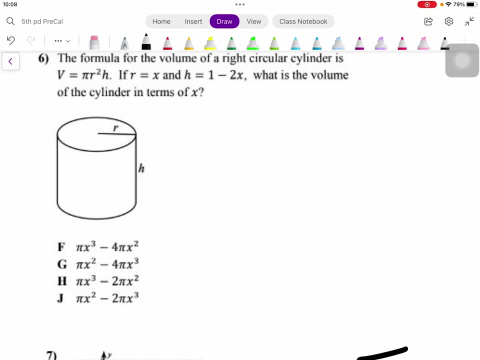 wording, you guys, So make sure that you read it and that you don't get confused. Okay, So we're almost done. We got two more questions. So what is the formula, or the formula of a volume? So we're going to be using this formula that they gave us. They gave us a few things right. They 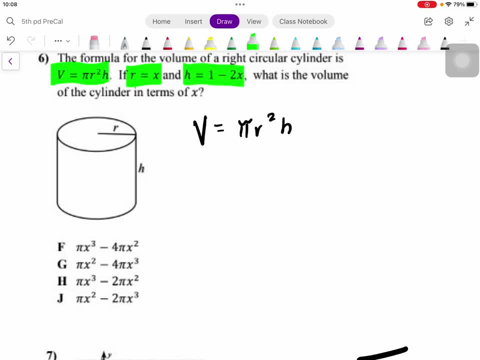 gave us our radius, and they also gave us the height. So we're going to go ahead and plug that in So V. we don't know. Pi is just a number, So we're just going to write it as pi And then we're. 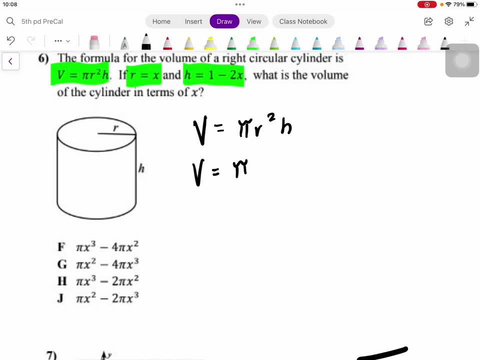 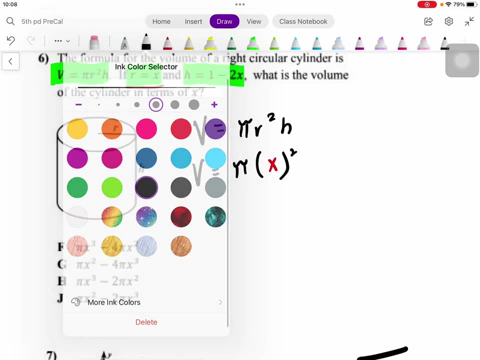 going to write it as pi, which is 3.14.. And then our radius is going to be- let's do it in a different color- is going to be X. And then here I have a squared. Now notice that I'm putting. 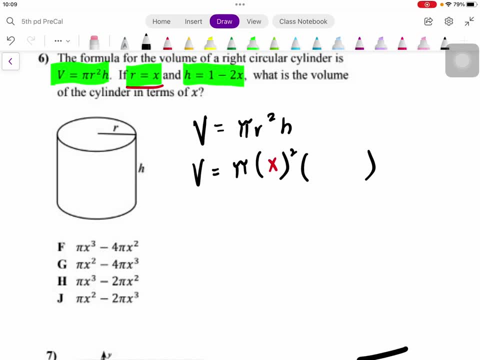 parentheses because I am multiplying, So it's probably best You don't have to if you don't want to, if you feel okay with it Now, H is going to be one minus two X. I'm definitely going to put that in parentheses because that is more than one term. Now I am going to erase the parentheses, for. 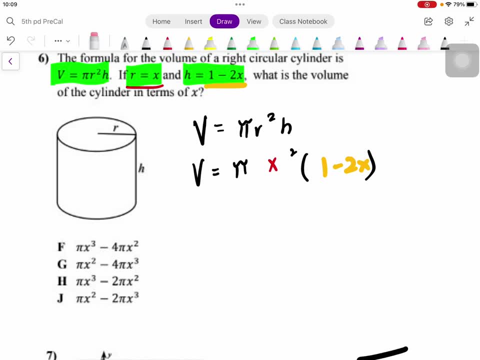 the X, because it's just X, And X to the power of two is just X to the power of two. All right, So now I need to simplify it. As you can see, your answer choices are simplified down over here, So we're going to take this whole entire. 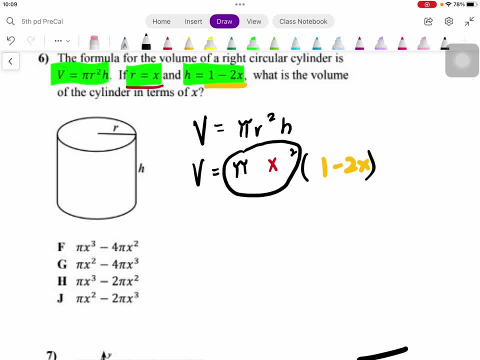 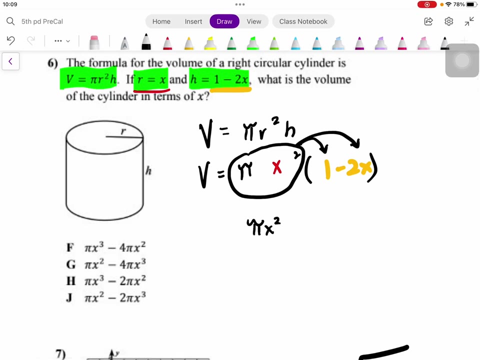 term right, Because pi is a number, X squared is just a variable with a power of two And I'm going to go ahead and distribute to each one of these because it is multiplying. So pi times X squared is just pi X squared. All right, Now pi X squared times negative two X. 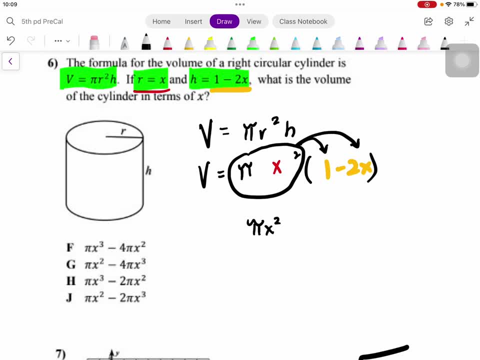 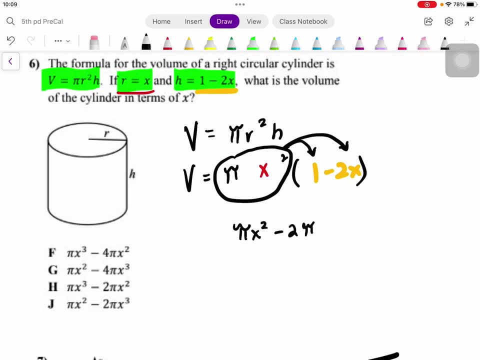 Well, think pi as just a number, and two is just. well, it's a number, right, So you're going to write it as negative two, You're going to attach the pi next to it. And then, of course, you multiply X, squared times X to the power of one. When you multiply X's together, you add the power, So it 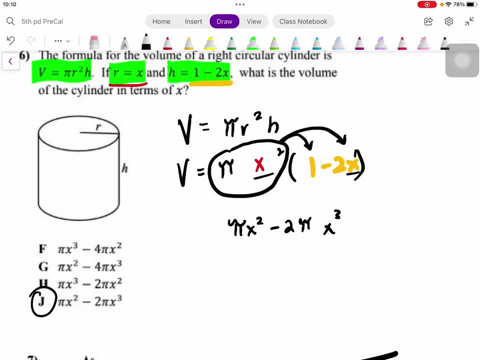 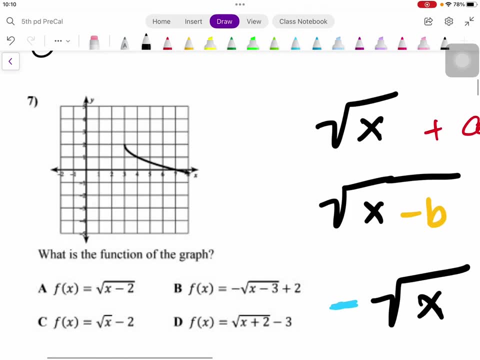 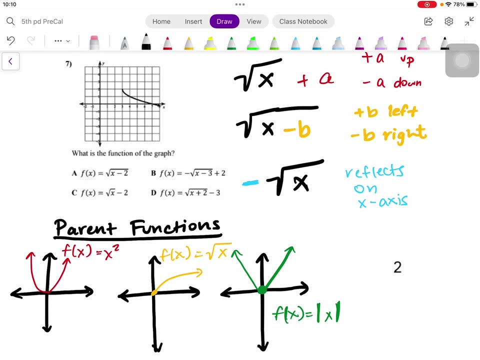 should be X to the power of three, So your answer choice should be: hold that. All right. Now our last one, last one- requires us to multiply, So we're going to take this whole entire term. Have a little bit of notes. So I wrote this prior. So if you will write this down because you are, 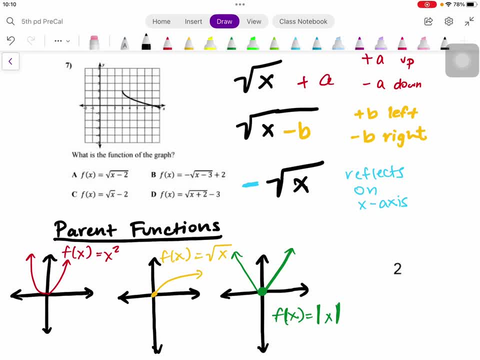 going to need this for for about three or four pages of your assignments. All right, So let's focus on parent functions. We have gone over parent functions in pre-calculus. Parent functions are the original right, Just like how your parents are the original. it's the same concept here. 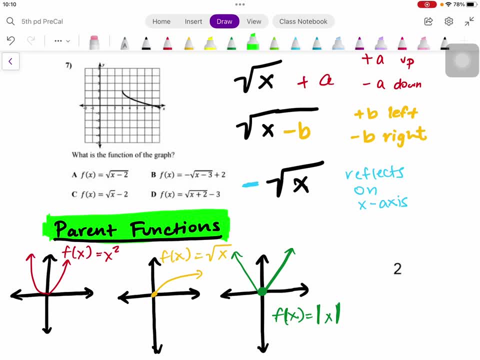 So the one in red is called X, to the power of two. It looks like a U, it's a parabola, it's a quadratic. Now the one on the one in the middle, the yellow one, that one is a square root of X. It's literally going through zero, zero and it just looks like. 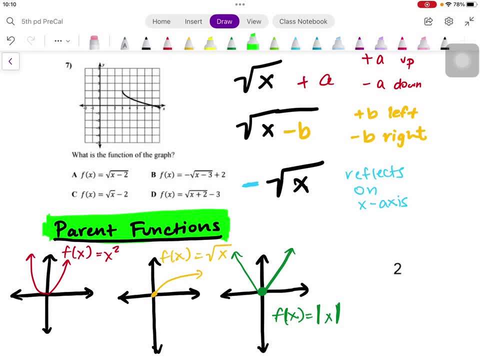 an arrow shooting out, All right. And the last parent function that we're also going to look at in the TSI also includes this absolute value of X, the one in green. it looks like a, B right Now we're also going to be looking at transformations of those three, So those 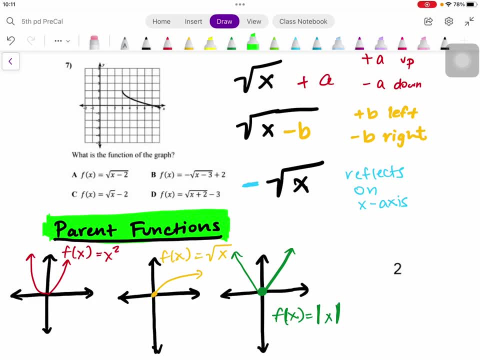 transformations of those three are the ones on the right-hand side, the one that says X squared plus A, X squared minus B and then negative X squared right. So you got those three. Now you're mainly going to look at the graph that's given below, or number seven, sorry, And as you can see that, one out of these. 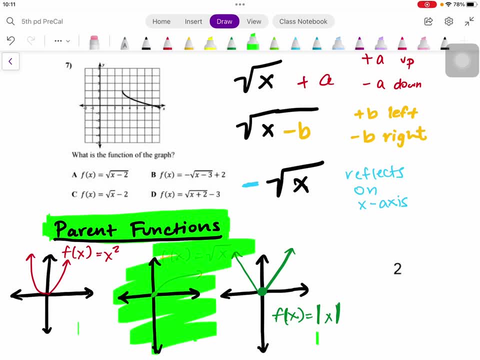 three right, It looks like it's going to be the X squared one right. That's why I chose X squared right. All right, So what? it looks like that it happened. it looks like it went. it shifted to the right, So it. 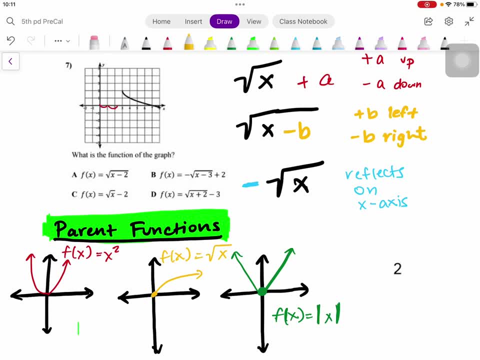 looked like it moved one, two. well, let me do that in yellow. So it moved one, two, three units. So when we're moving to the left, it's going to be a plus three right. So it's really going to. 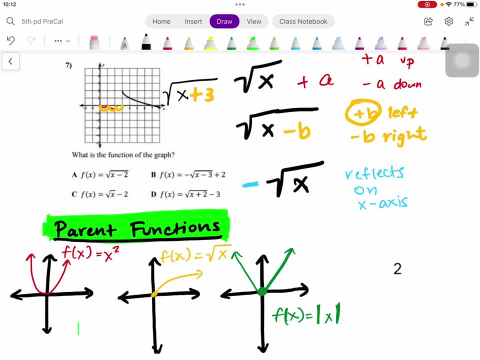 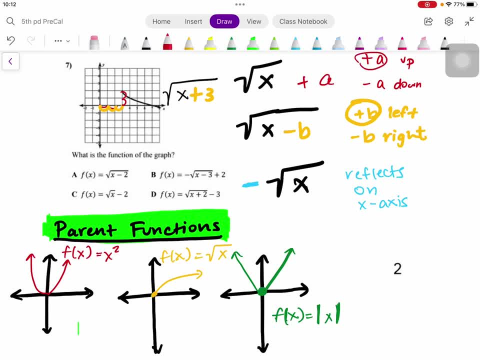 two. Now, when you're going up, you're going to be adding something outside of the square root, just like how it is here in the example. So it's going to be a plus two outside the square root. Now, as you can see, here it's going from here. it's going shooting up like this, but when it's